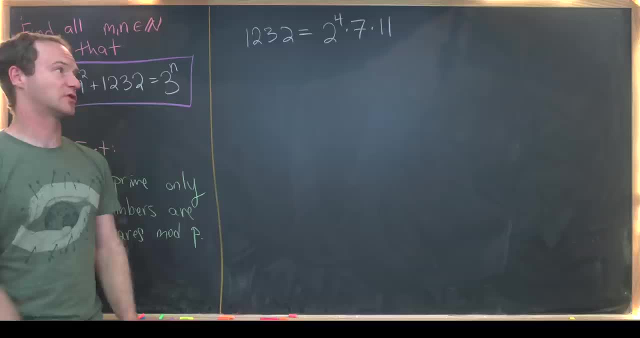 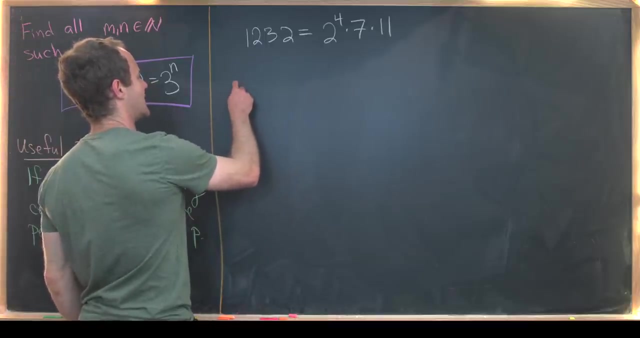 super helpful, And that's because everything is a perfect square mod 2.. So we'll probably want to reduce mod 7 or 11 to get an idea for the possible values of n. So let's do that. So the first thing that I'll do is make a list of x and then x squared mod 2.. So let's do that. So let's do that. 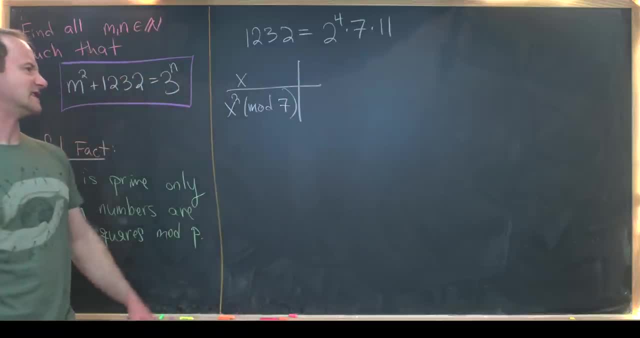 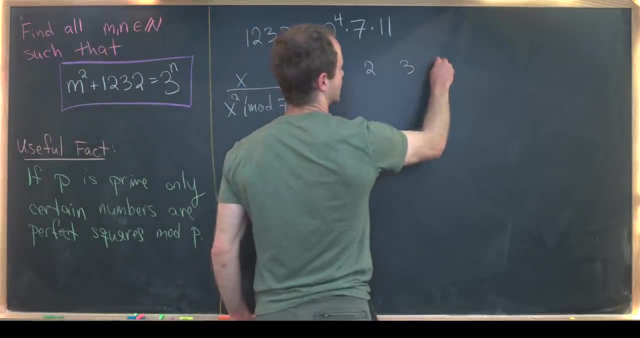 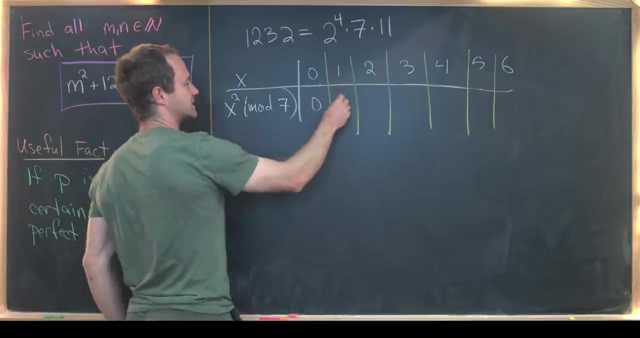 mod 7.. Just to get an idea of what the perfect squares, mod 7 are: Okay, so we'll do 0, 1,, 2,, 3,, 4, 5, 6.. Okay so, 0 squared is obviously 0.. 1 squared is 1.. 2 squared is 4.. 3 squared: well, that's going to be. 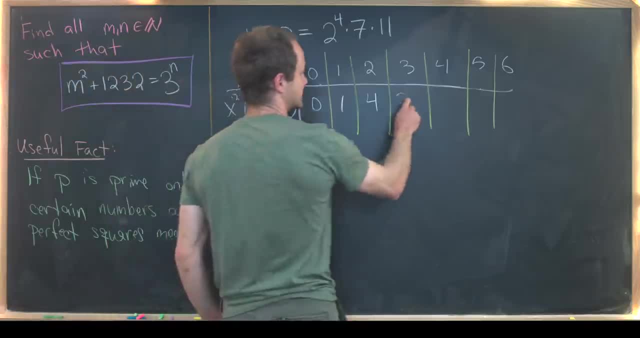 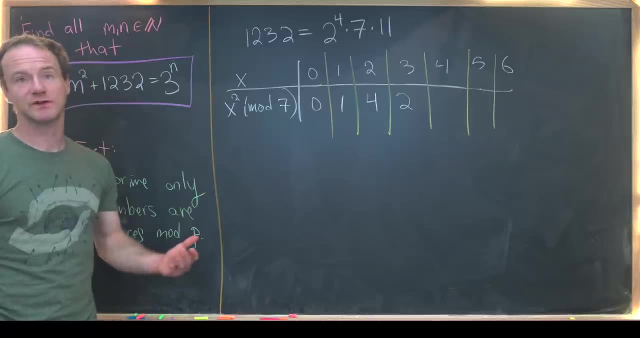 9. But if we reduce 9 mod 7, we get 2.. 4 squared is 16. But if we reduce 16 mod 7, we also get 2. Because 16 is 2 more than 14. And then 5 squared will be, let's see, 25. But 25 is 4 more than 21. So that is 4. And then 6 will. 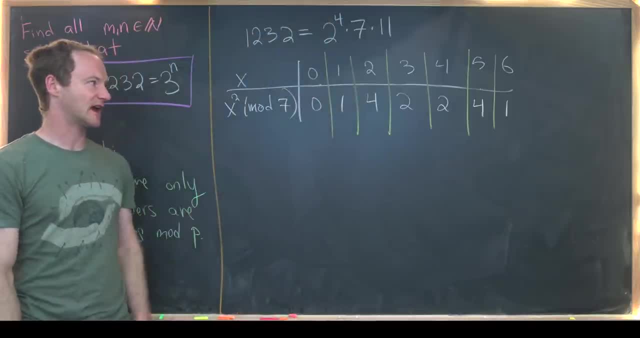 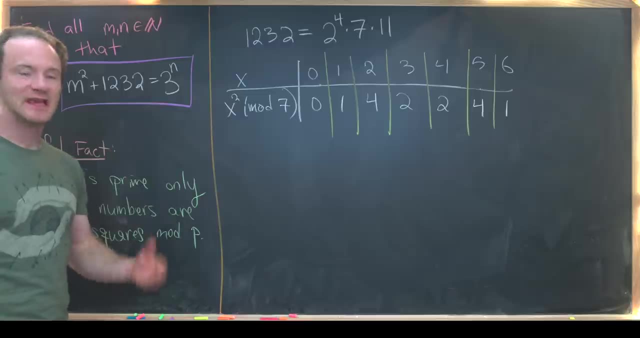 be 1. We can see that super quickly because 6 is negative 1 mod 7. And then negative 1 squared is kind of obviously positive 1.. Now, maybe in parallel, let's look at the powers of 3 mod 7.. 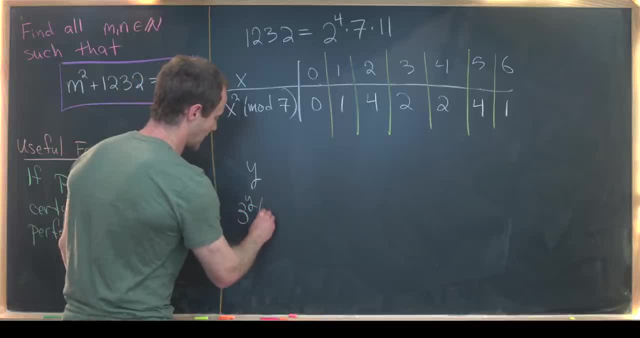 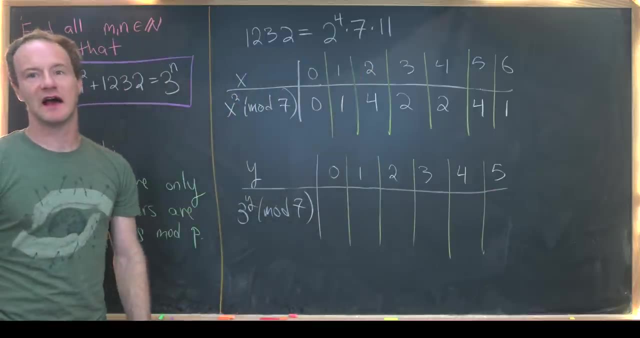 So I'll say y, and then 3 to the y, mod 7.. So let's make a chart for that as well. Now notice, I've only gone out to 5 in my chart, Because in fact I know that 3 to the 6 is the same thing as 3 to the 7. 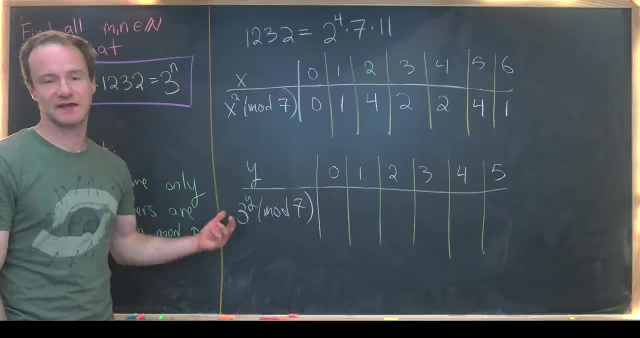 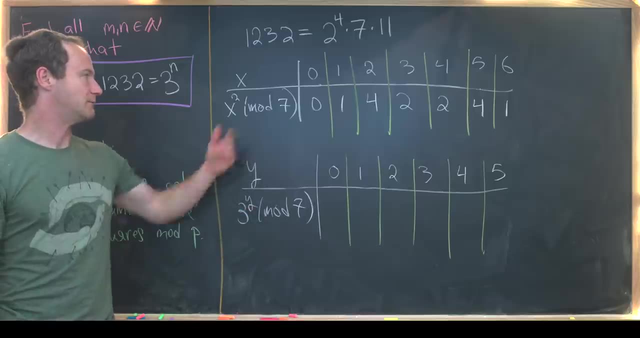 minus 1.. And by Fermat's little theorem we know that's congruent to 1 mod 7. So we don't really need to go further than that. So just to kind of reiterate what's happening more generally, If your base is being calculated, mod 7.. 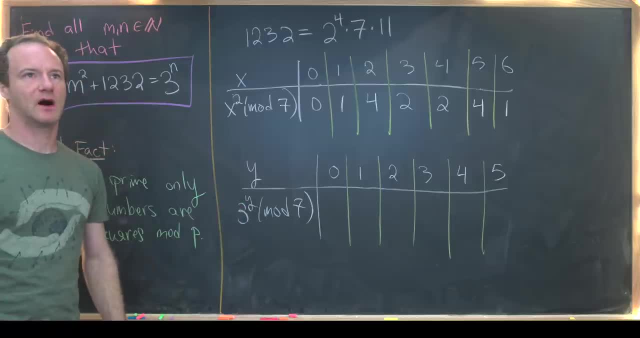 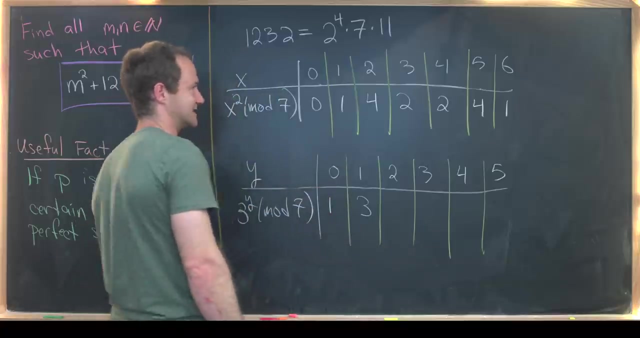 mod n, Then your exponent is being calculated mod phi of n, Where that's Euler's totient function. But phi of a prime number is just that prime number minus 1.. Okay, anyway, let's get to this: 3 to the 0 is 1.. 3 to the 1 is 3.. 3 squared is 9.. But like in our previous calculation, 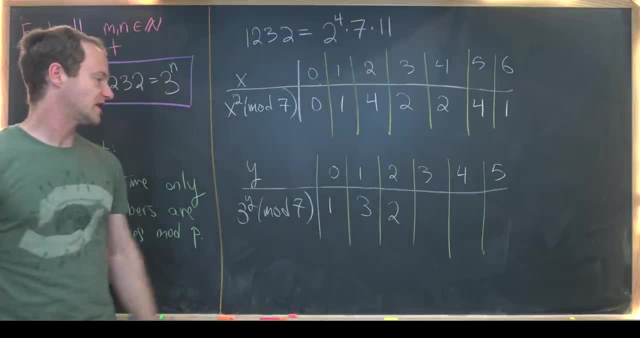 9 is the same thing as 2.. 3 cubed is 27.. Notice: 27 is 1 less than 28.. And so that makes 1 less than 28.. And so that makes 1 less than 28.. And so that makes 1 less than 28.. 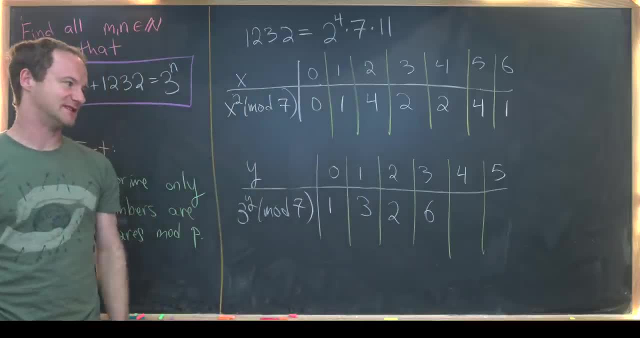 6. 1 less than 28 means it's negative 1.. But negative 1 is the same thing as 6.. 3 to the 4th is 81.. Well, let's see, 81 is 4 more than 77. So that means this thing is 4.. And then 3 to the 5th. 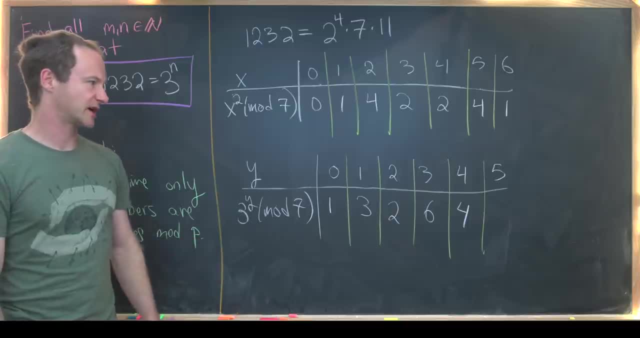 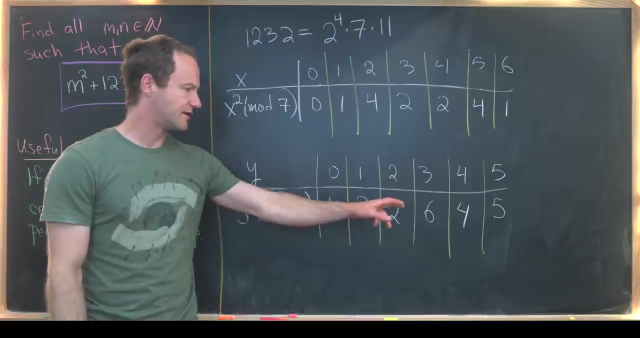 Well, that's 243.. But let's use a trick. That's the same thing as 3 to the 4th times 3.. So that's the same thing as 3 times 4 mod 7.. That's 12 mod 7.. In other words, it is 5.. Well, notice that we get all of the numbers except for 0.. 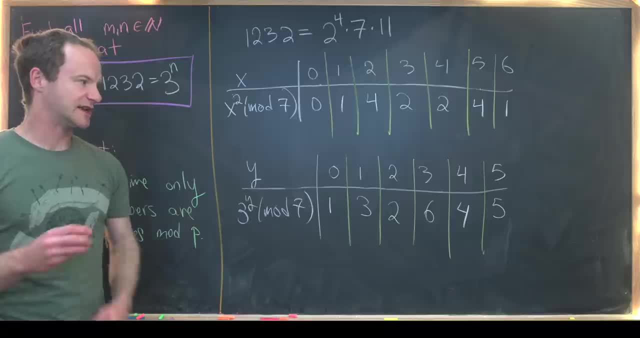 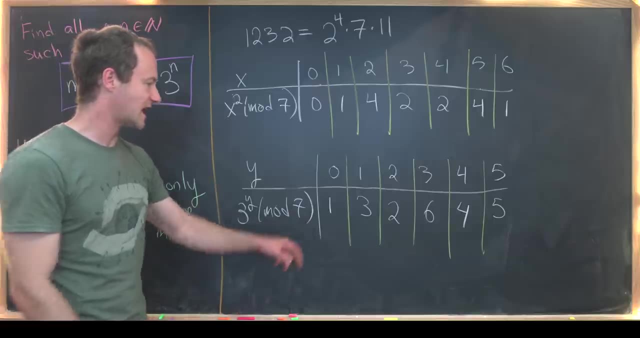 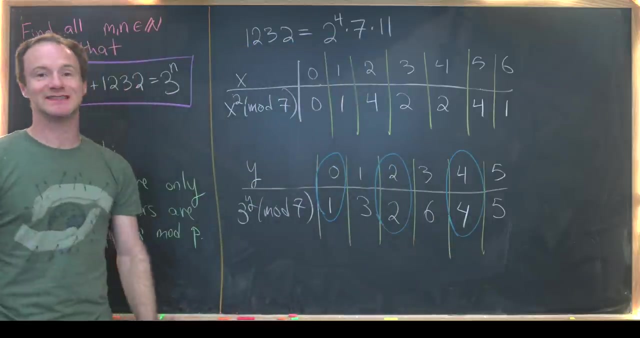 That actually makes 3 something called a primitive root- Again something you learn in elementary number theory class. But now what's important to point out is that the only time we get perfect squares on this list of powers of 3 is when the exponent is even Notice. that gives us a 1,, a 2,. 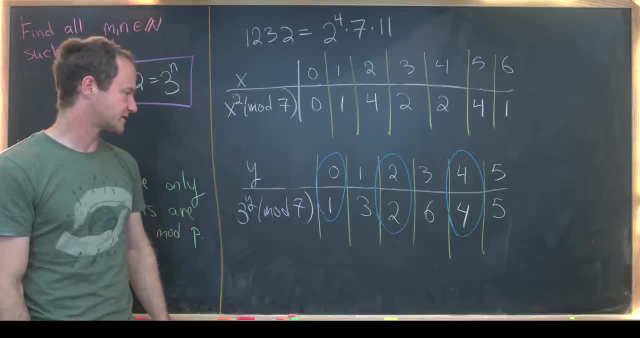 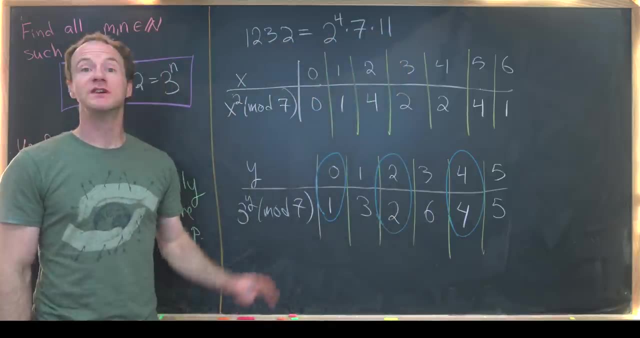 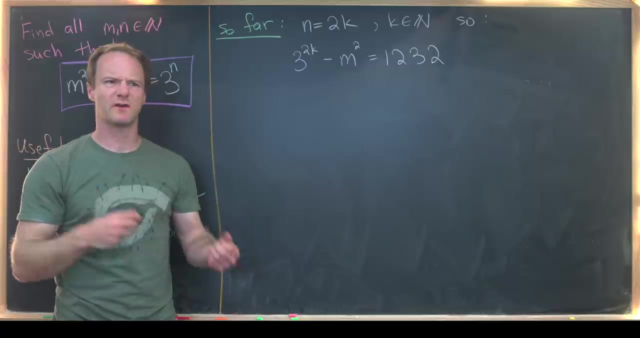 or a 4. So that's 1 mod 7.. But those are the only perfect squares. So from that we immediately see that this n, this exponent here, is even. So, let's clean up the board and then we'll attack it using that data, Using a modular arithmetic argument involving quadratic residues. 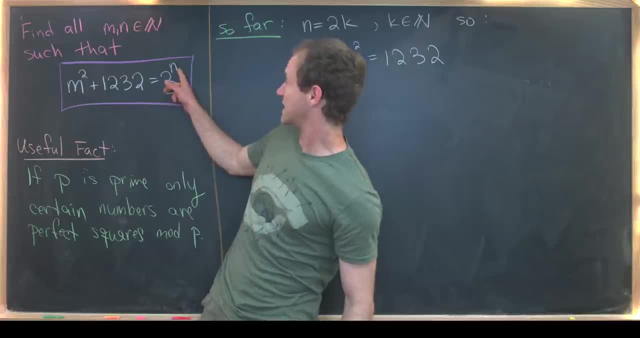 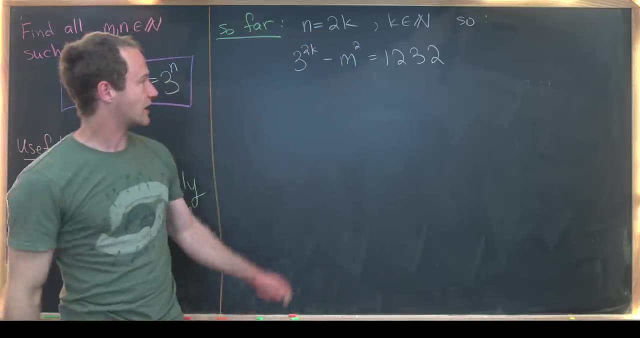 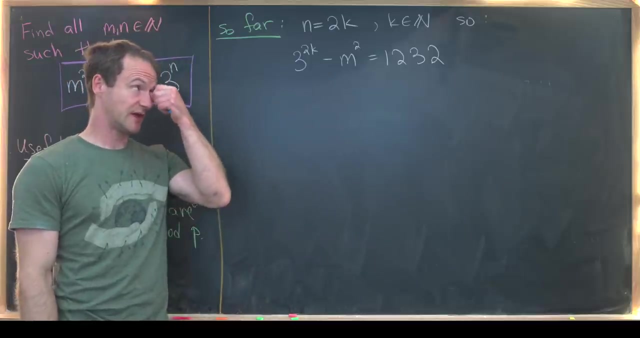 and stuff like that. we realized on the last board that this exponent of 3 needed to be even. So that means we can take this purple boxed equation and rewrite it as: 3 to the 2k minus m squared is equal to 1,232.. So there, I've replaced my n with 2k. Now that we've. 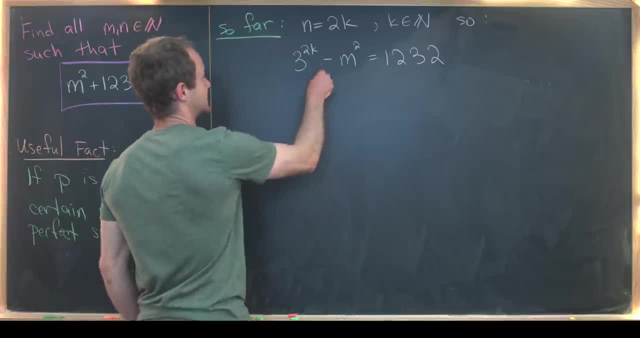 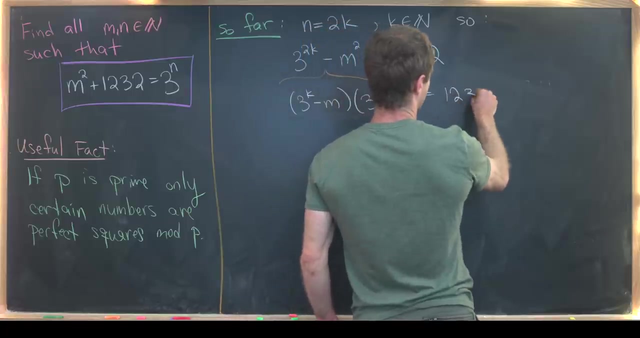 got it in this form. this is just begging us to factor this left hand side of the equation using a difference of squares factorization, So that'll be: 3 to the k minus m times 3 to the k plus m equals 1232.. 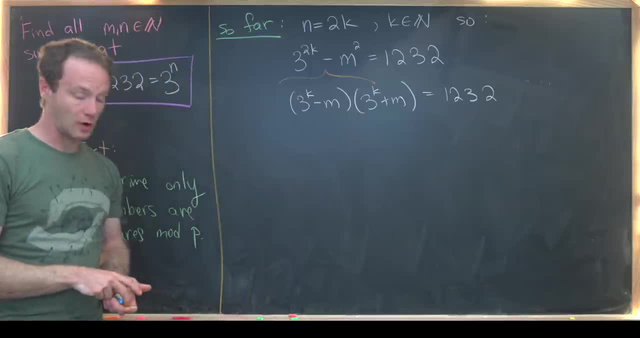 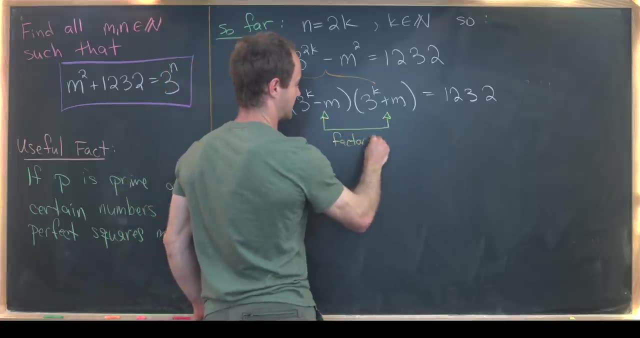 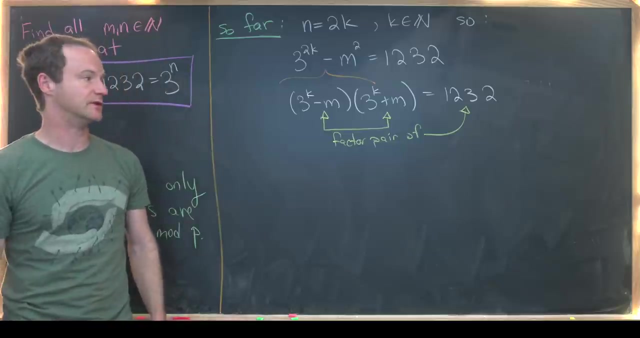 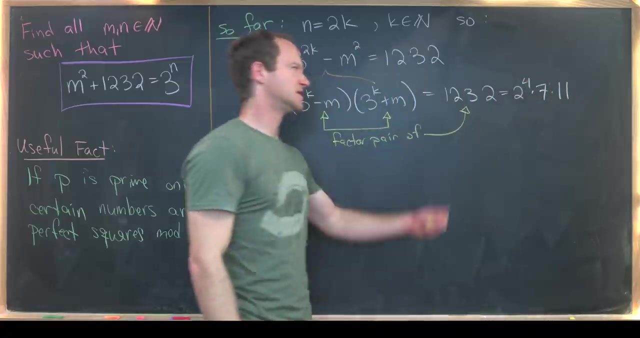 But everything involved on this left hand side is a whole number. So that means what we have constructed is a factor pair of this thing over here on the right hand side, this 1232.. But let's recall, 1232 was equal to 2 to the 4 times 7 times 11.. So the fact that 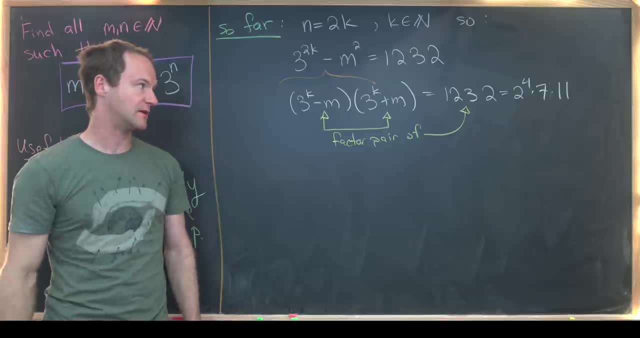 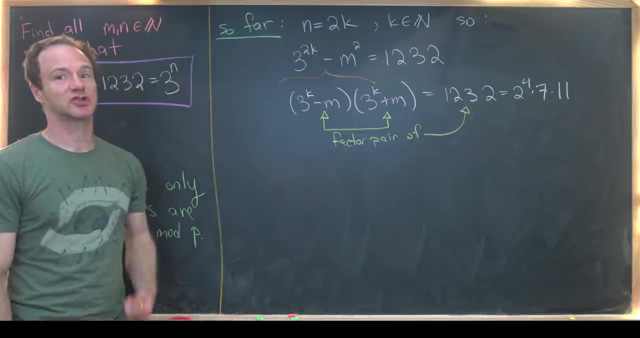 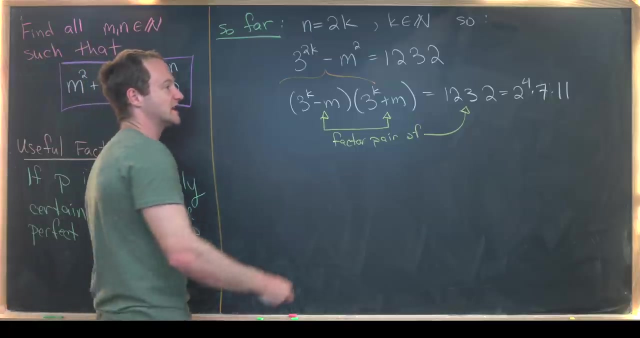 we've got that fourth exponent of 2, along with two more primes, mean that we've got a ton of factor pairs for this 1232. So we've got to think about a trick for pairing it down. And maybe the thing to notice is that if we sum these two we'll actually get twice. 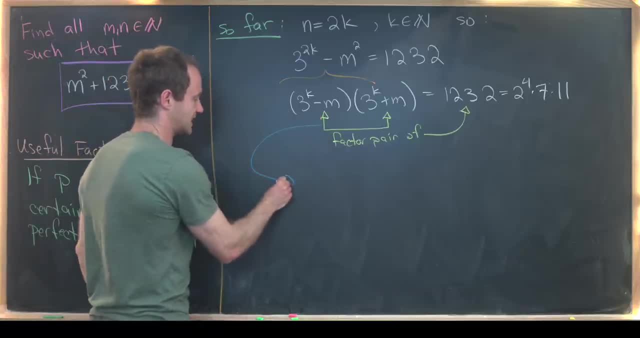 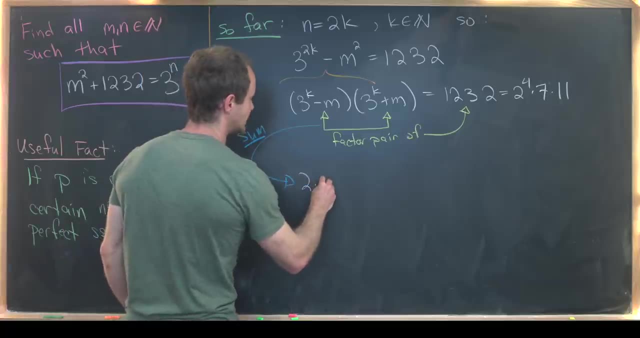 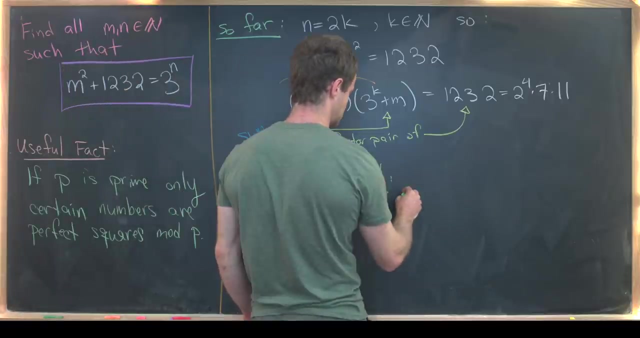 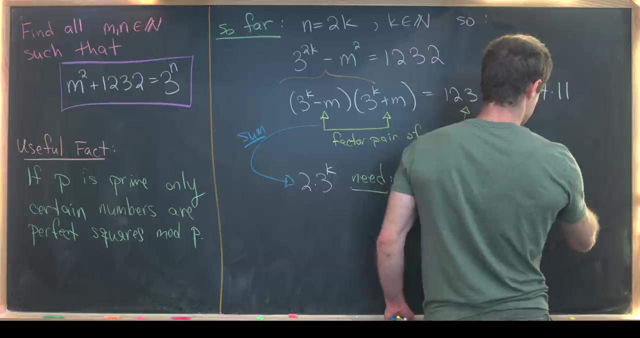 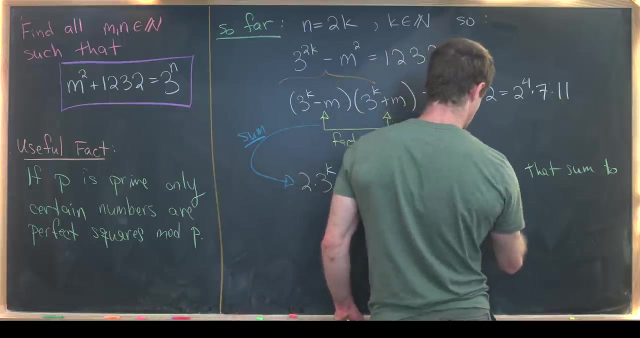 a power of 3.. So let's maybe do that. So let's sum these two factor pairs or this factor pair, and notice that we get 2 times 3 to the k. So that means what we need are factors of 1232 that sum to 2 times 3 to the k. for some, 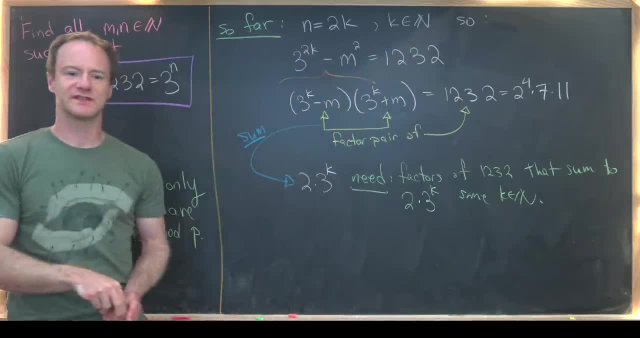 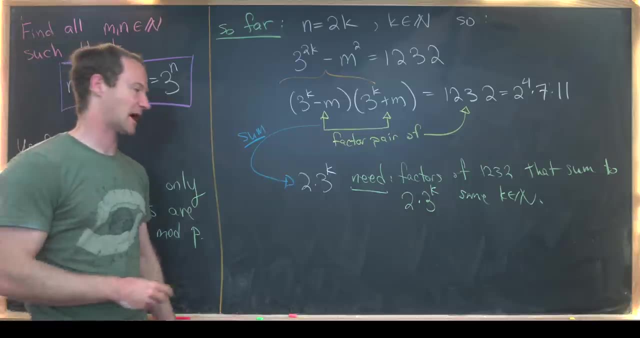 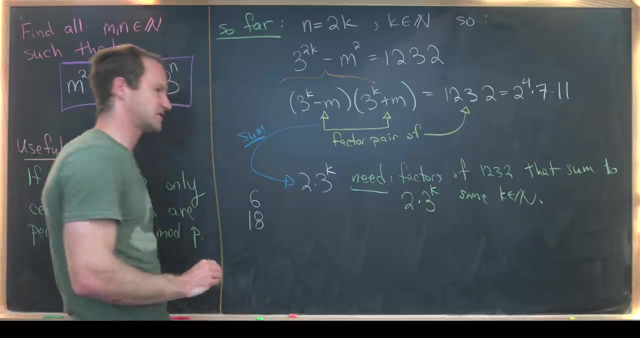 natural number k. In other words, it's got to be twice a power of 3.. So let's just make a list of all of the numbers that are twice a power of 3.. So we've got 6.. That's going to be 2 times 3 to the first. We've got 18.. That's 2 times. 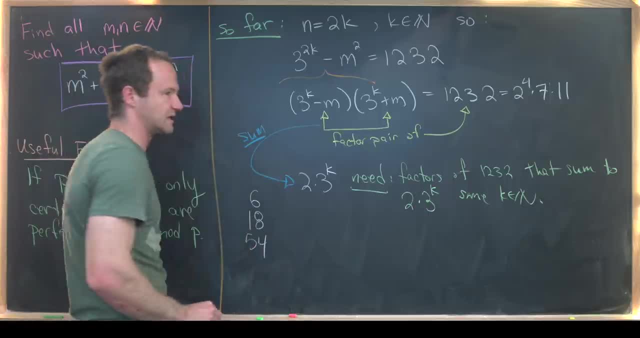 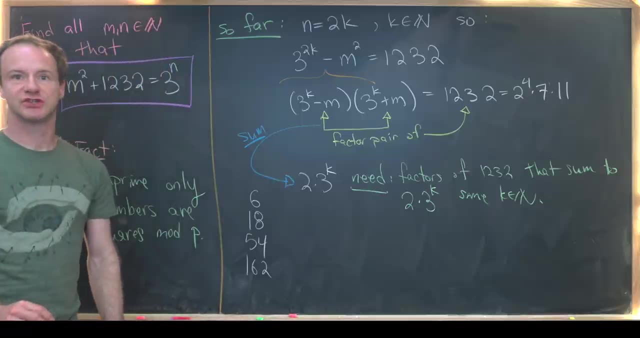 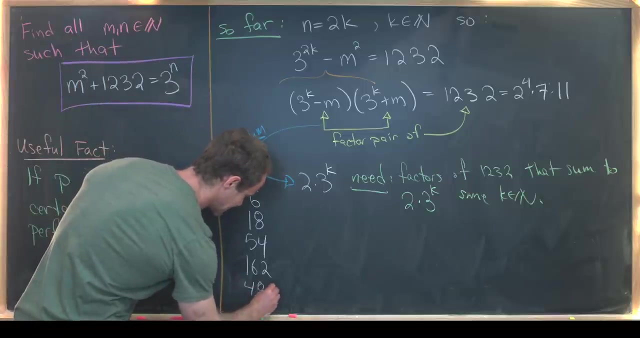 3 squared, We've got 54.. That's 2 times 27,, which is 2 times 3. cubed, We've got 162, which is 2 times 3 to the 4, 2 times 81.. And then, finally, we've got 486, which is 2 times 3. 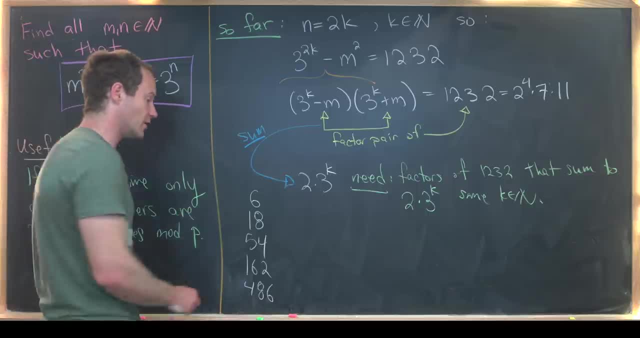 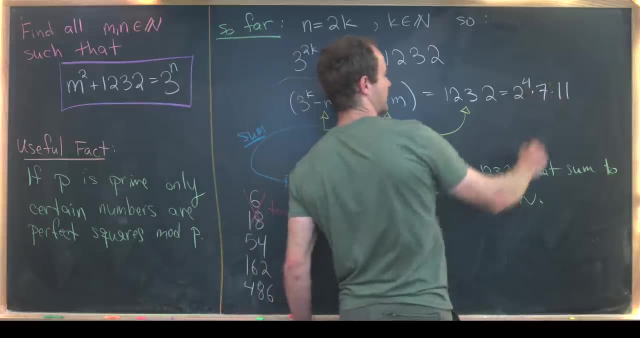 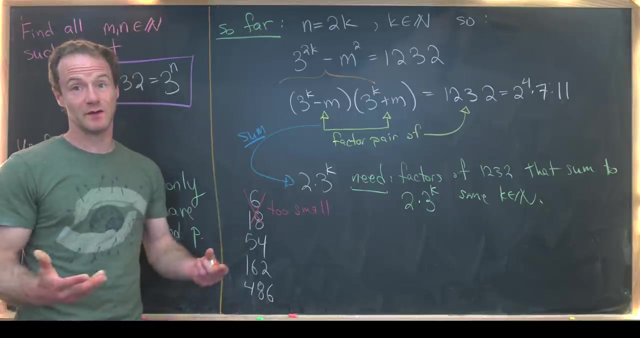 to the 5.. Immediately, I want to notice that these first two are too small, And I think that's pretty clear by the fact that we've got a bunch of factors over here, and one of them is 7 and one of them is 11.. So I think the smallest sum you could get would be evenly. 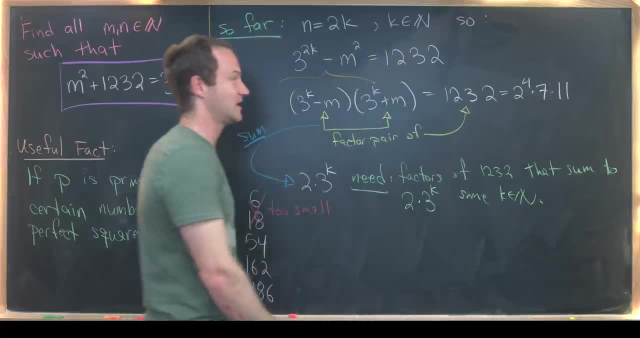 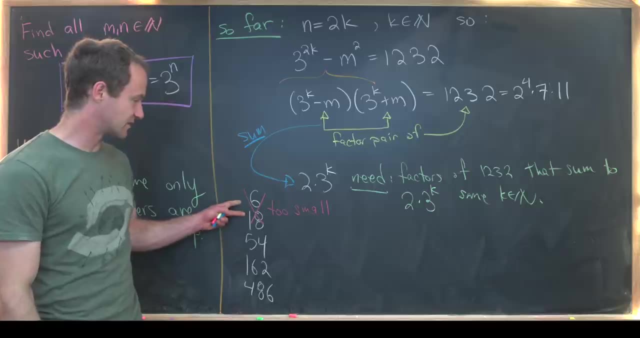 distributing these twos over the 7 and 11.. So in other words, it would be something like 28 plus 44. But 28 plus 44 is clearly bigger than 7 times 18.. But I think it's pretty clear that if you've got a factor pair of 1232, you're never going. 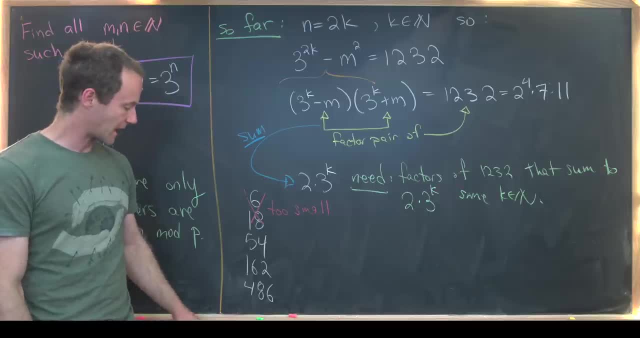 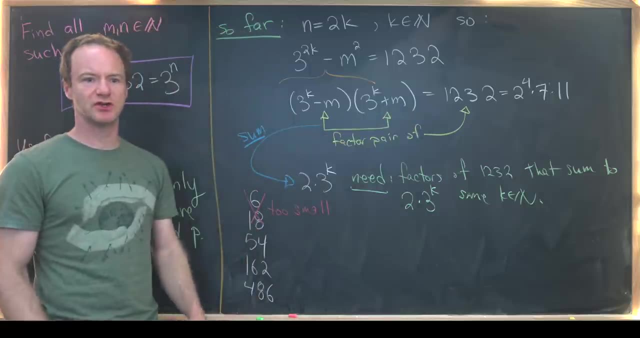 to be able to get 7 or 18 out of it. Okay, well, let's move on to 486.. So let's think about the ways to factor 1232 with numbers that are as large as possible to maybe achieve this 486.. 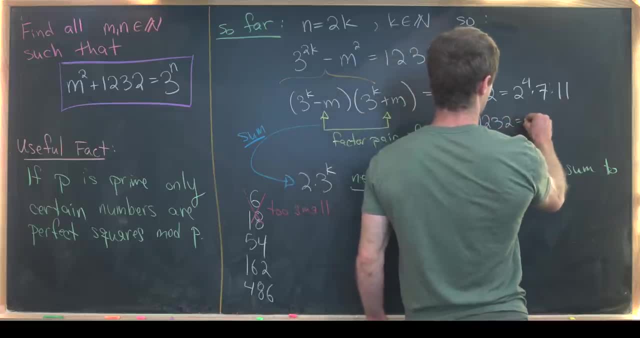 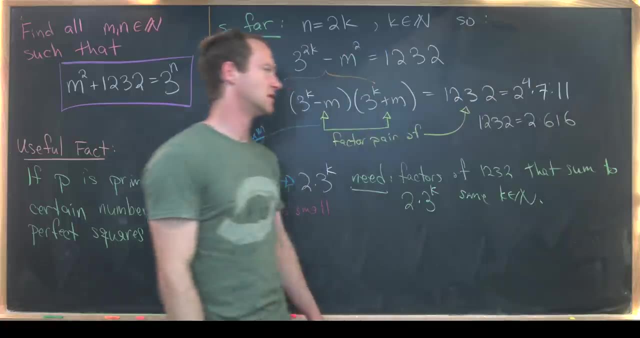 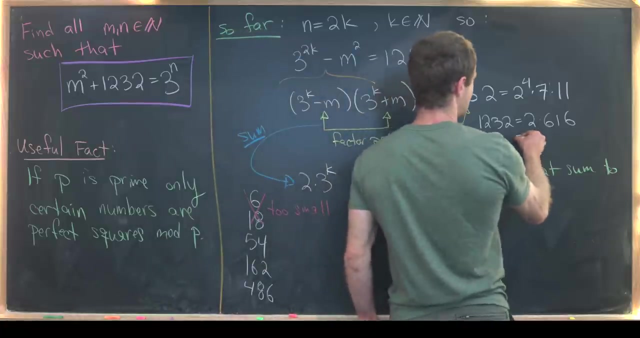 Well, one way would be to write 1232 as 2 times something, And in fact it's 2 times 660.. But notice, if we add 2 and 616, we do not get 486.. It's too big. Well, maybe the next. 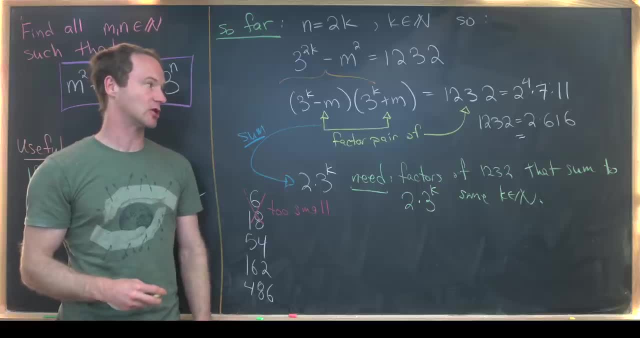 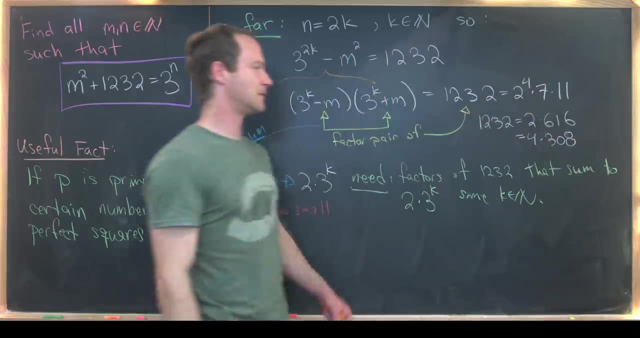 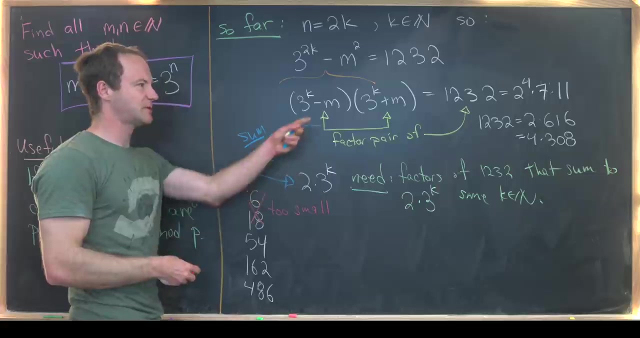 way to do it, which would produce the second largest value of the sum would be 4 times 308, that factorization. But now 4 plus 308 is too small: 486.. So I think just by looking at those two cases, 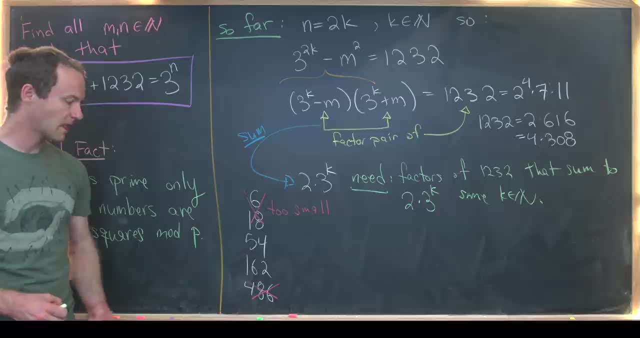 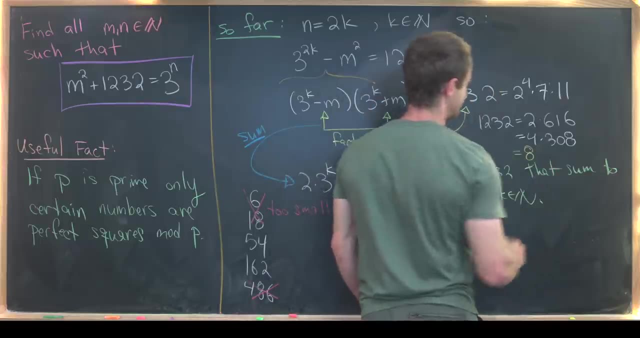 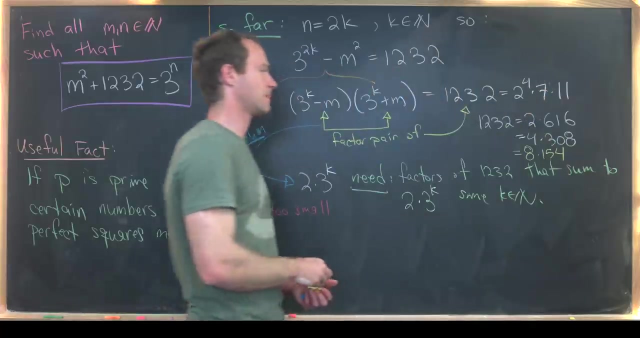 we see that this one is not as big. Okay, Okay, It's not possible, So let's move on to this 162.. And we'll notice that 162 works, And that's by taking the factorization of 1232 of 8 times 154.. 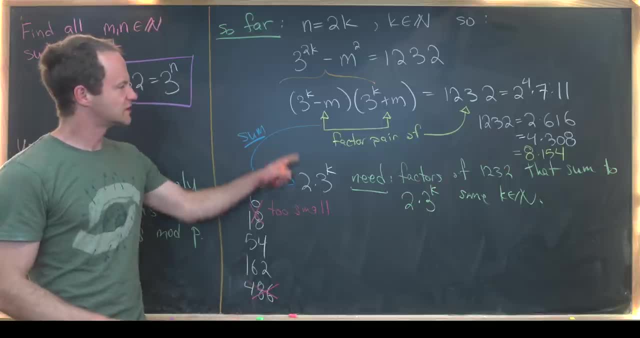 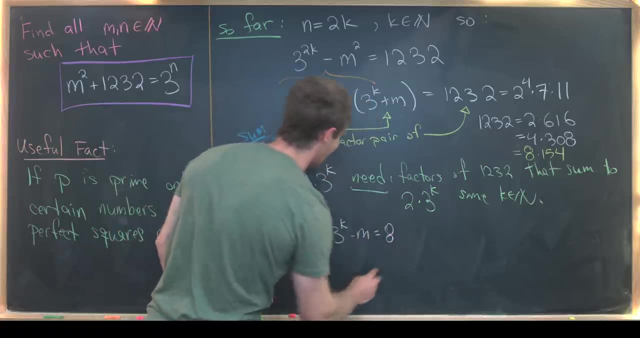 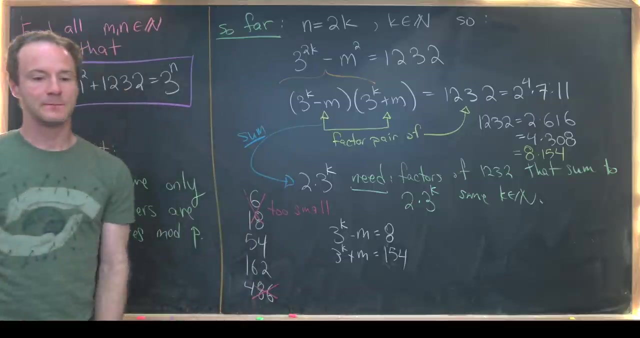 And noticing that 8 plus 154 is 162.. So what does that say about these factor pairs? That means that 3 to the k minus m is going to be equal to 8.. And 3 to the k plus m is going to be equal to 154.. 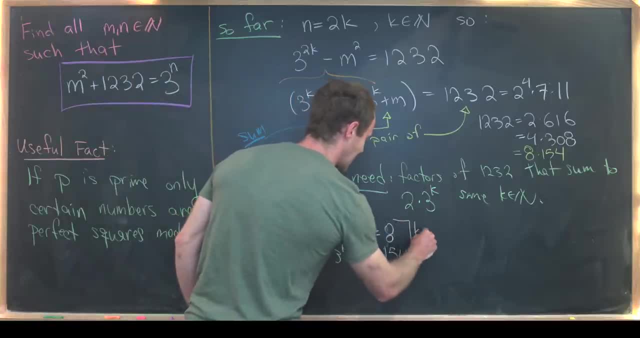 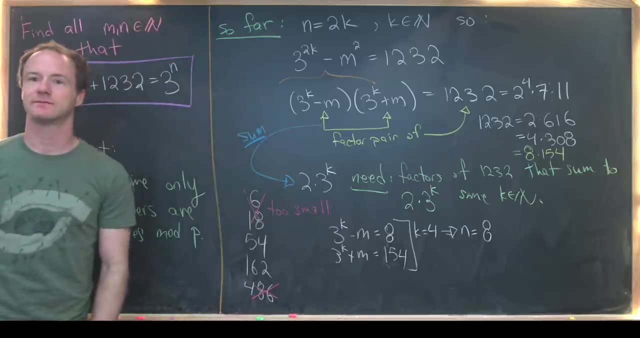 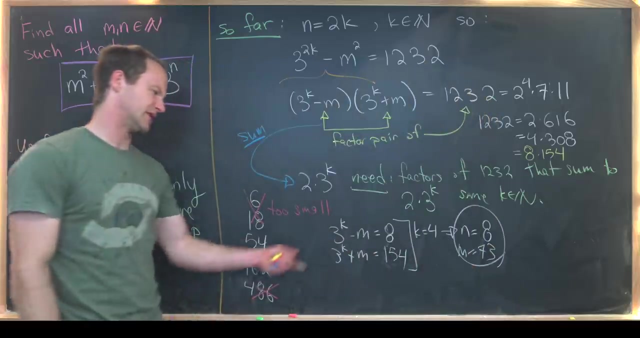 Okay. So if you play this game, you'll see that k must be equal to 4, which means our original n, which was 2k, will be equal to 8.. And then m will be equal to 73.. And so that's just from solving this fairly standard system of equations. 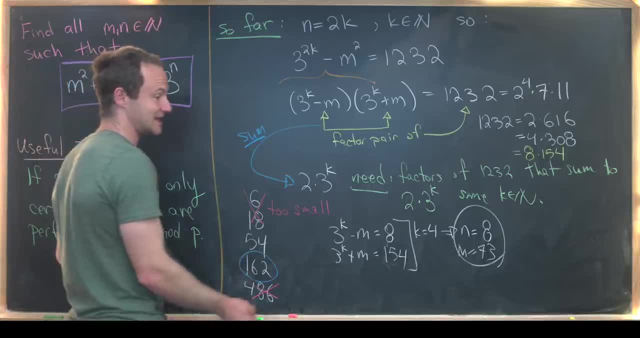 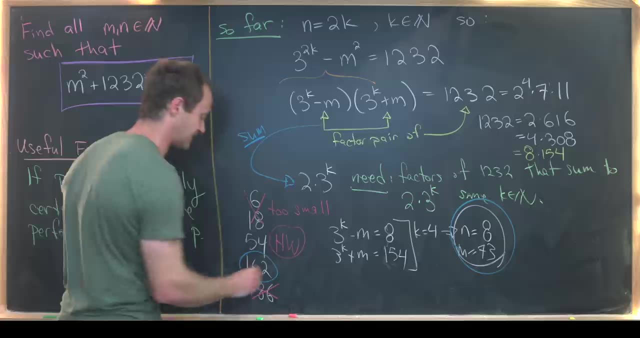 Okay, So that means that this possibility did yield a solution, which was the solution to the solution which we have over here, And then maybe I'll leave it as homework for you guys to check if this 54 gives us a second solution, or maybe this one is the only solution.